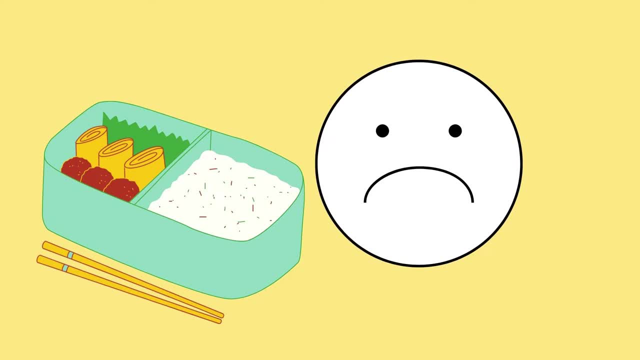 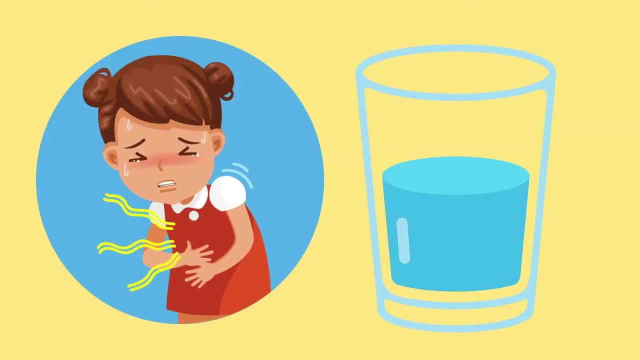 She was upset and closed the lunch box. Then she went outside to play with her friends. By the time she reached back home, her tummy was burning. She did not understand what was going on. She was also feeling very tired. She drank a lot of water, but it did not seem to help much. 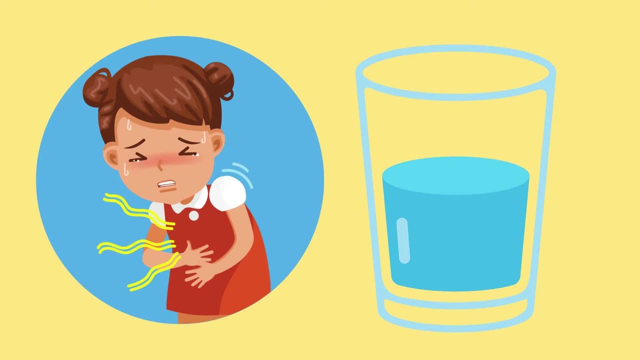 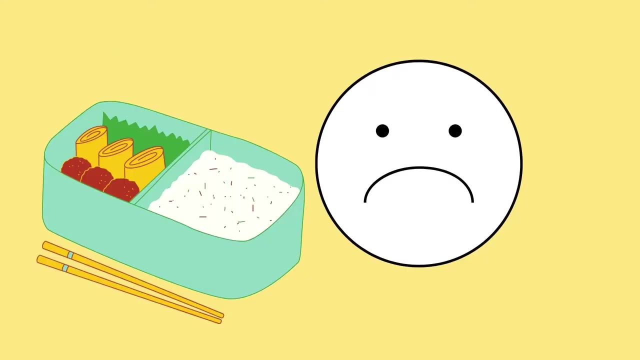 Her mom offered her some yummy food, but she could barely eat a few mouthful. Something was wrong. Then her mom took her lunch box out for being cleaned and noticed that she had not even had a bit of her food. She asked what had happened and Moon said it was not her favorite food. 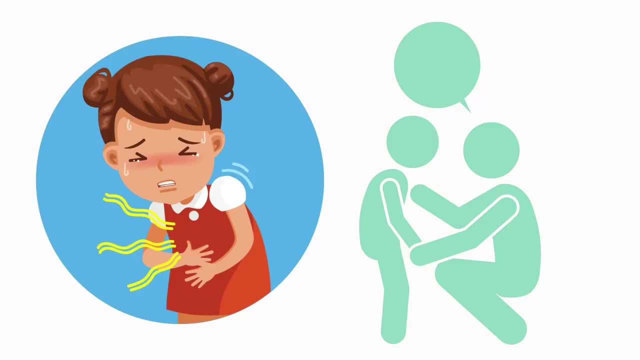 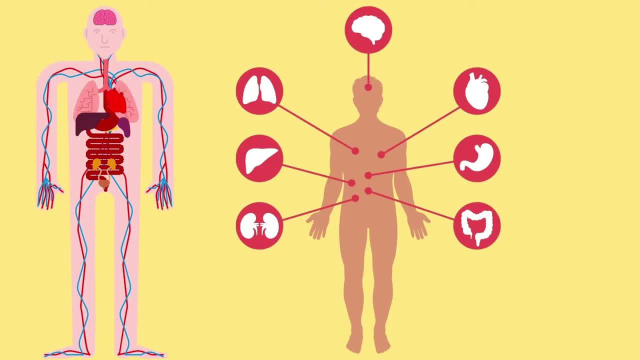 Mom told Moon. Do you know what, Moon? The human body has many organs. Each of these organs help us live and they all must keep working for us to be all right and to stay alive. If you do not eat one time, you are starving: not just your tummy, but all the other organs as well. 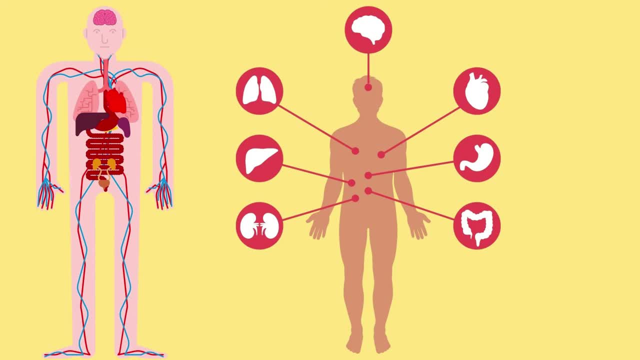 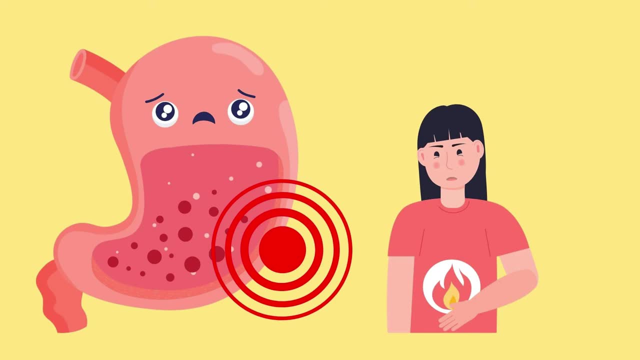 They are not getting enough energy to do their work. This, in turn, makes you tired. Also, your tummy has acids to break down your food. The acids will continue to be there even when there is no more food. This will make you feel gassy and uncomfortable. 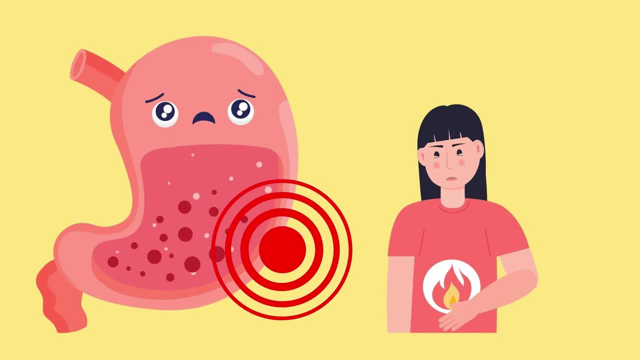 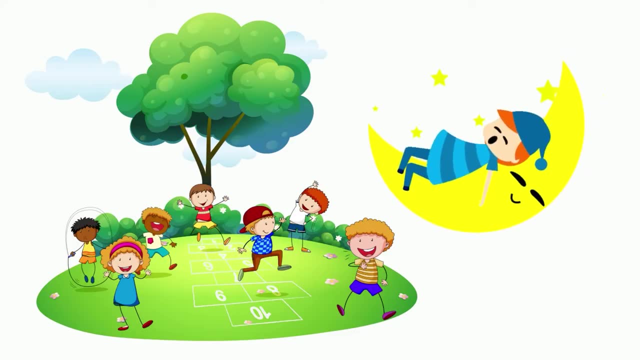 Do you understand why it is important to eat when you are hungry, Even if it is not your favorite vegetable? you must eat to let your body work normally. You also need energy to play, study, walk, run and do every activity. You even need energy to sleep. 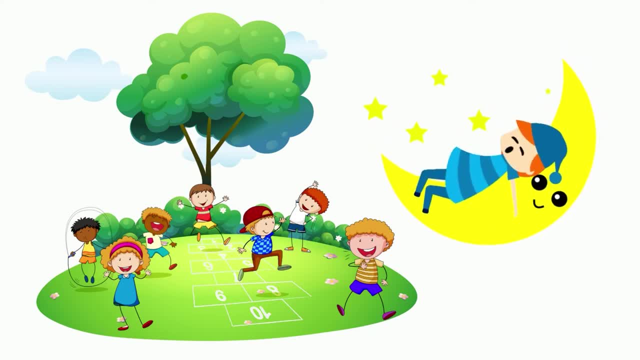 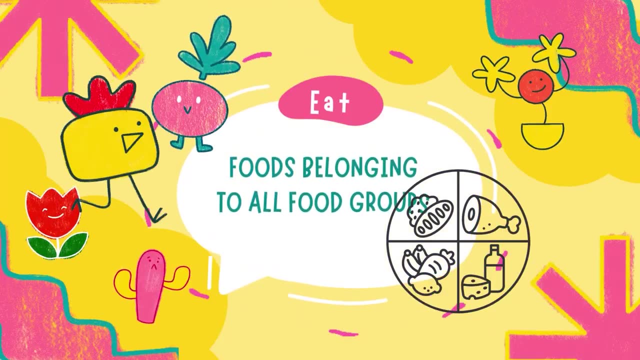 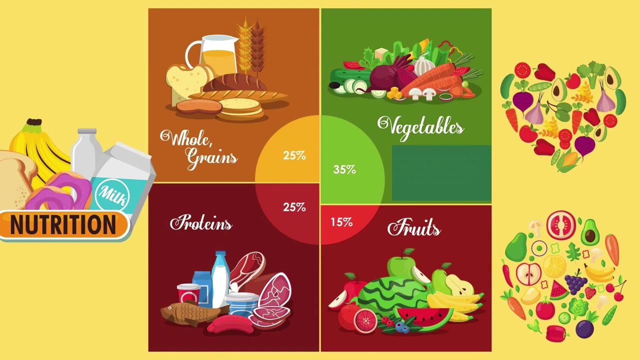 Your body is like a machine. It needs enough fuel to work properly. You also need the nutrients from food to grow, like the rest of your friends, If you do not eat all kinds of foods, you will not get all kinds of nutrients. While some nutrients help to grow in height, others help to grow healthy muscles.